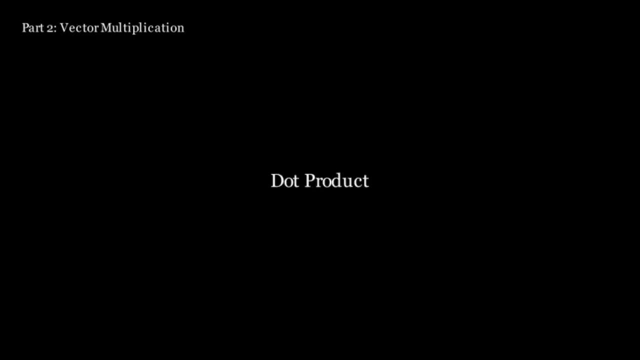 What's different with vectors, though, is that there are different types of multiplication. The first is called the dot product, and it's the most intuitive. Just multiply each of the numbers in a vector by the corresponding one in the other vector, add the results up, and that's your dot product. This may seem arbitrary, but there exists an. 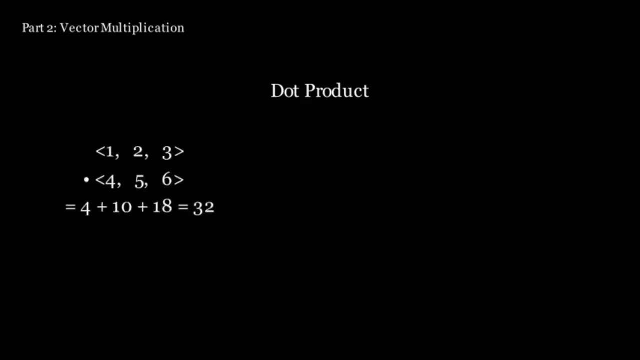 interesting connection between dot products and the spatial relationship between two vectors. Two perpendicular or orthogonal as they're called in 3D space vectors will always have a dot product of zero. For two parallel vectors, the dot product is equal to the 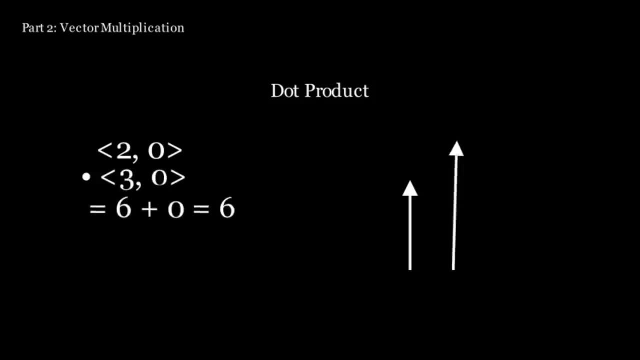 product of the magnitude of the two vectors. This property extends to become the following formula, where theta is the angle between the vectors u and v and the double absolute values mean magnitude of The cross product is the other main way of multiplying vectors. This product can be: 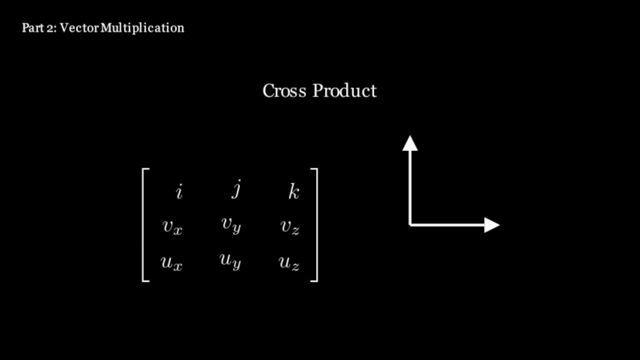 expressed as the determinant of this matrix, where i, j and k are the unit vectors in each of the x, y and z directions respectively, And v and u are the vector being multiplied. The cross product also has an interesting property: It always generates a vector that 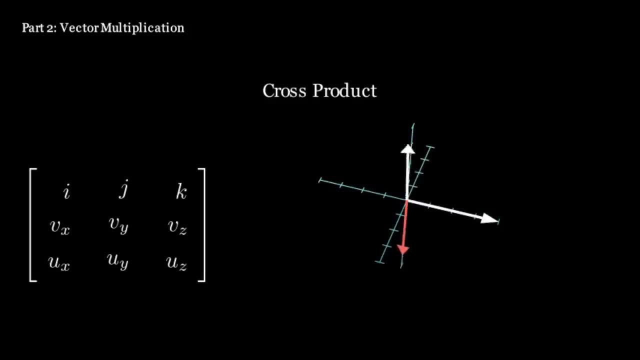 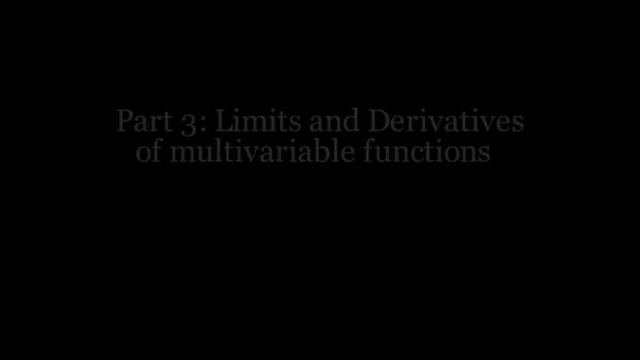 is orthogonal or perpendicular to the two vectors being multiplied. Part 3. Limits and derivatives of multivariable functions. Just like with 2D functions where we approach an x value, we can take the limit of a 3D function where we approach a value on the x- y. 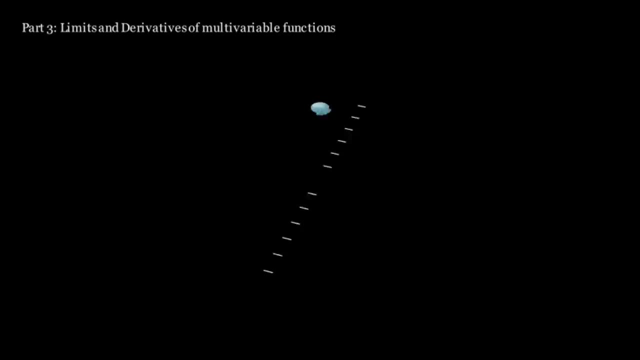 y plane. Using these limits, we can also define a derivative, just like one would in 2D. One thing to note is that there are infinitely many derivatives of a 3D function. at a certain point, since there are infinitely many directions one can go in, Each of these are called directional. 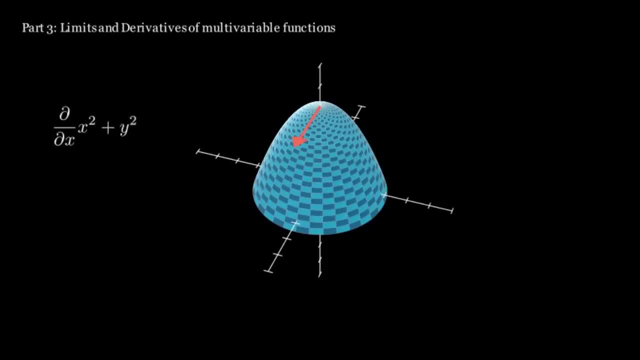 derivatives. Also, taking the partial derivative with respect to x gives us the derivative in the positive x direction, and differentiating with respect to y gives us the derivative in the positive y direction. The gradient is a generalization of this Gradient and a point is a vector, with components being the derivative in the. 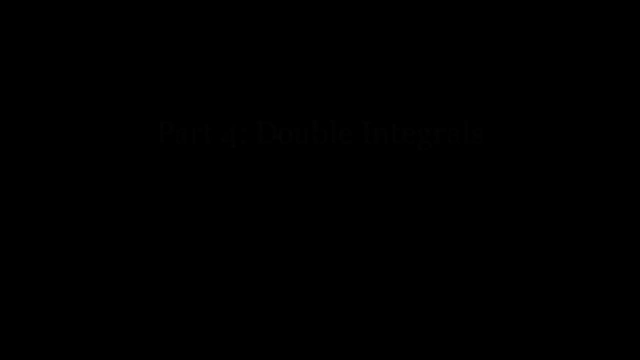 x-direction and y-direction. Part 4. Double Integrals: Just like we defined differentiation, integrals also exist with multivariable functions. When doing a double integral, instead of finding the area under a function, we're finding the volume under it. To do this, first do an integral in the x-direction and then integrate that. 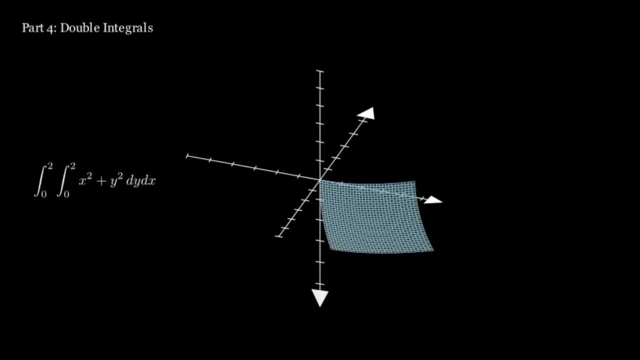 area a second time over the y-direction, effectively extruding it. But that isn't all. we can do with double integrals. You can also integrate over a non-rectangular region. Instead of having the bounds of the integrals be numbers, they can be functions. 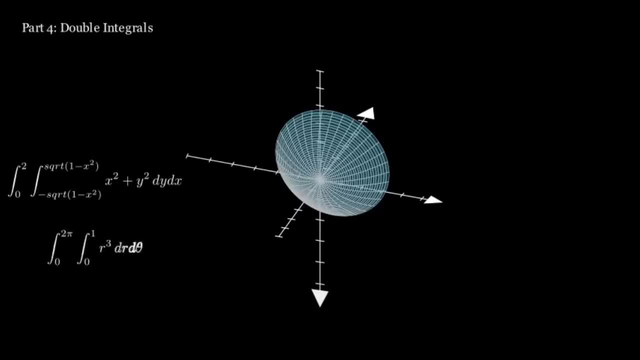 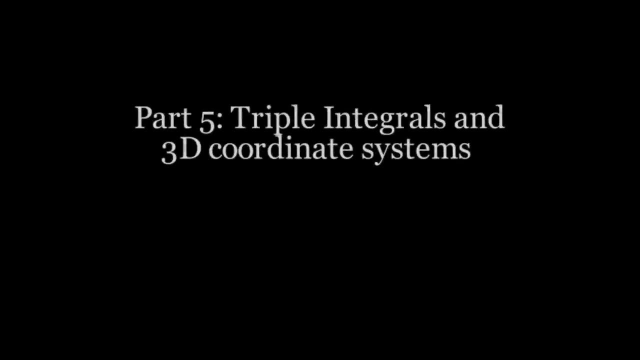 We can also use polar coordinates for double integrals where, instead of making an integral dy dx, it is dr d theta. Notice that the polar equation we're integrating is r cubed instead of r squared. More on that later, Part 5.. Triple Integrals and 3D Coordinate Systems. 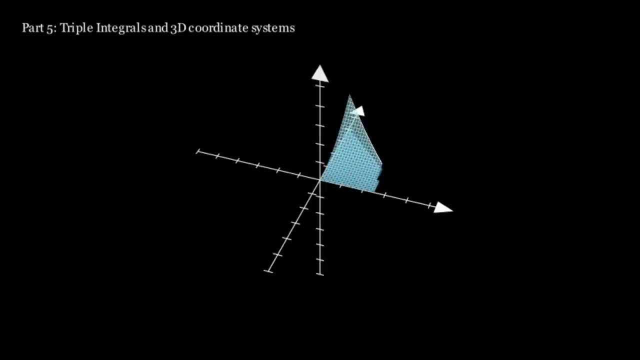 Triple integrals can also be integrated over a non-rectangular region. For example, if we want to find the area under a function, we can also integrate over a non-rectangular region. With triple integrals. we can integrate any 3D region, as long as we can define it with. 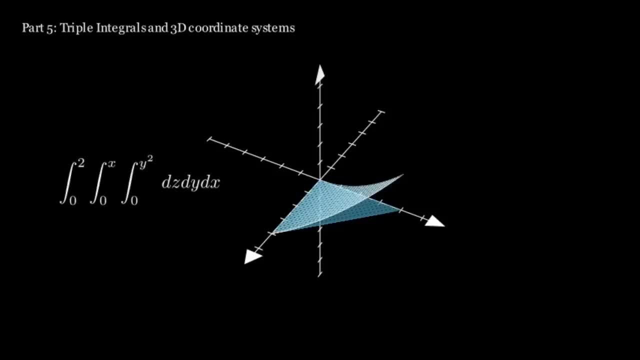 three different boundaries instead of two. Here, x goes from zero to two, y goes from zero to x, forming a triangular base, and z goes from zero to y, squared, creating a sort of parabolic shape. Triple integrals can also be used for finding things like average temperature, where we 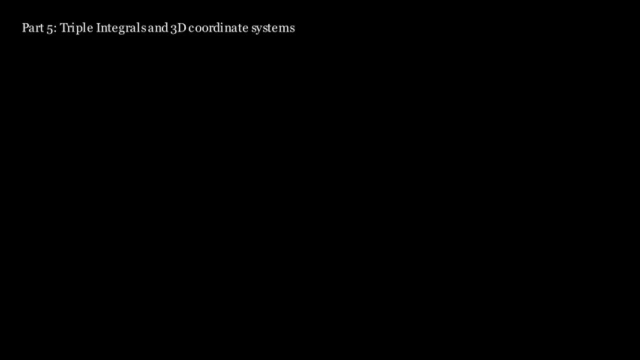 would integrate the temperature function over a 3D surface to find the average temperature. When doing a double integral, sometimes it's easier to convert to polar coordinates. Likewise, there is an analogous system in 3D space, Or rather two analogous systems, cylindrical. 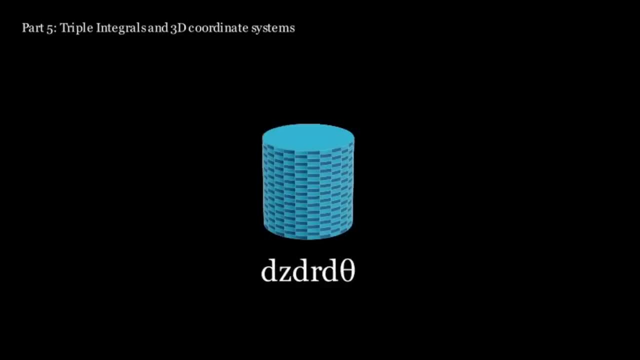 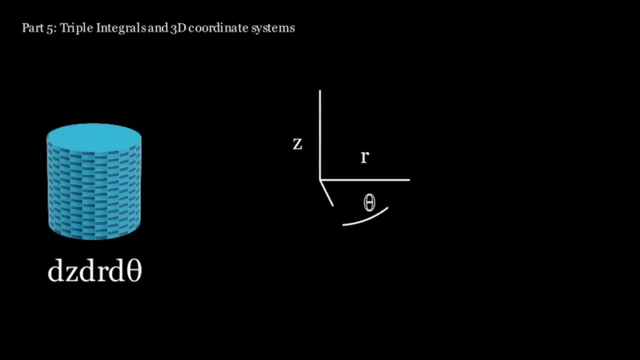 and spherical coordinates. In cylindrical coordinates there is a radius, r a z coordinate and an angle. theta. In spherical coordinates, there is a radius and two angles: Rho is the 3D distance from the origin, Phi is the angle from the vertical axis and theta is the angle. 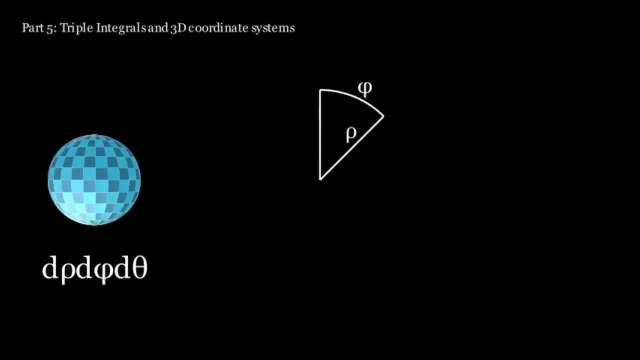 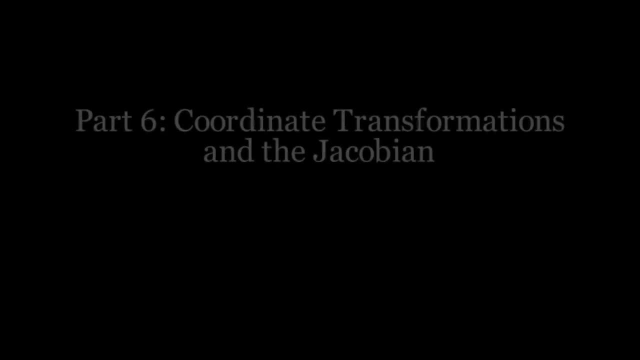 from the vertical axis. In spherical coordinates there is a radius and two angles. Rho is the 3D distance from the origin, Phi is the angle from the vertical line which passes through the origin, And theta works just like in polar. 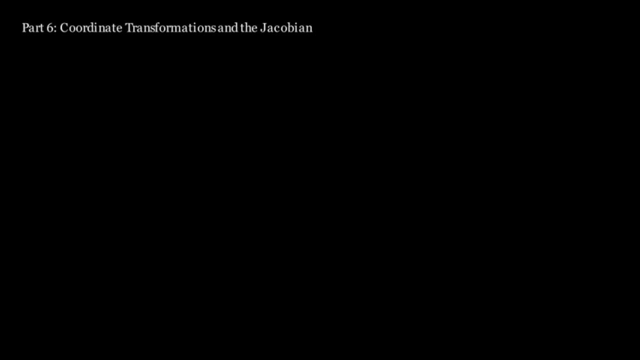 Part 6. Coordinate Transformations and the Jacobian. There is actually an infinite number of coordinate systems, not just the ones described previously. Any coordinate system can be defined as x equals g of uv and y equals h of uv. As an example, in polar coordinates this is x equals r cosine theta and y equals r sine theta. This 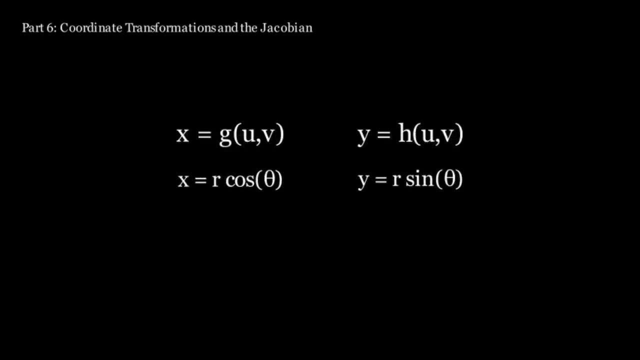 is a very simple equation, but it can also be defined as x equals g of uv and y equals h of uv. As an example, in polar coordinates this is: x equals r cosine theta and y equals r sine theta When changing an integral from one coordinate system to another one. 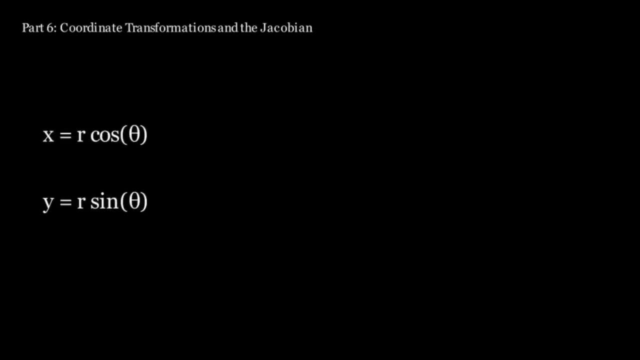 must add a certain function- j- the Jacobian- to the inside of the integral to account for the distortion that switching coordinate systems creates. Let's do this for the example of a double integral shown earlier. Here we can see the Jacobian being added to the inside. 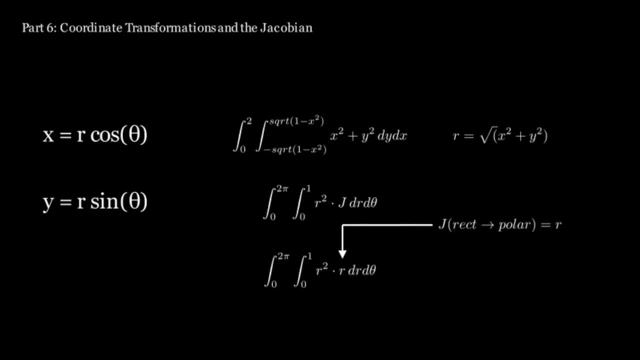 of the integral. What I just said is basically an oversimplification of the reason behind the Jacobian, and the real reason involves a ton of cool math with matrices where the Jacobian is a determinant, but that could be an entire video of its 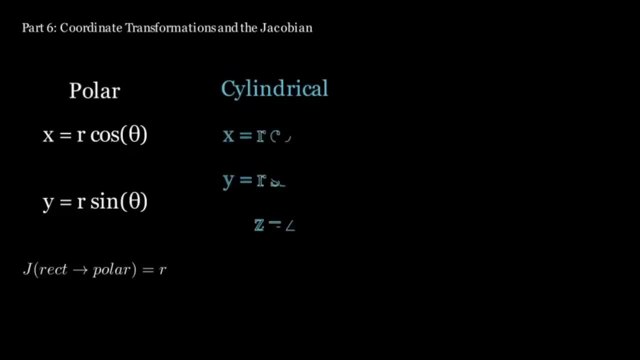 own. Anyways, here are the transformations needed to convert to polar, cylindrical and spherical coordinates. Part 7. Vector fields, scalar fields and line integrals. A vector field is an assignment of a vector to each point in a plane or space. A scalar? 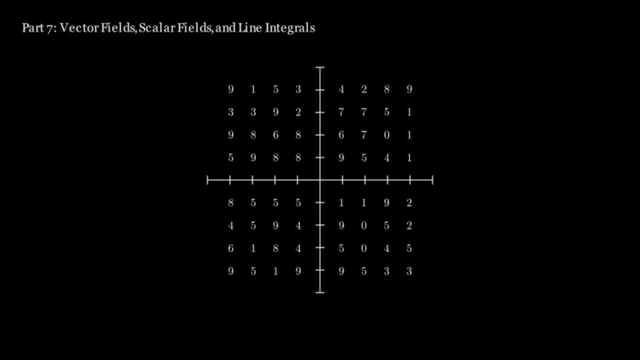 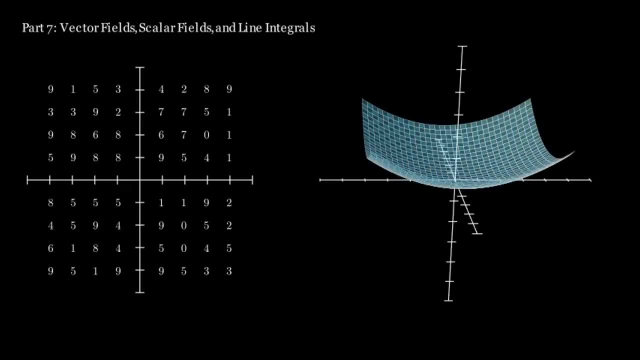 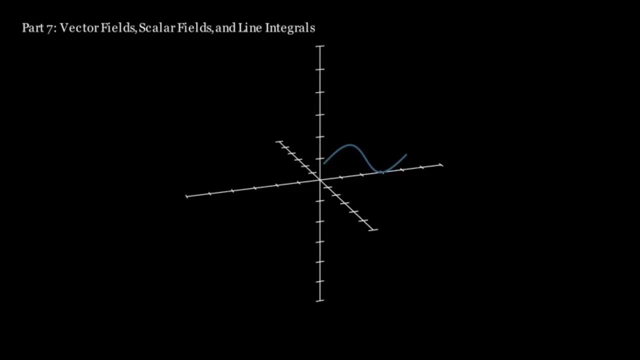 field is essentially that, but with regular numbers, aka scalars. Think of these as 3D surfaces above a 2D plane. In a way, they're essentially the same thing as 3D functions. When you take an integral in Calc 1, the integral is always done on a flat surface. think sheet of paper. 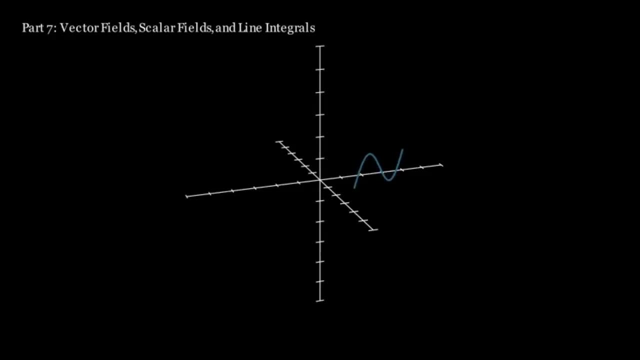 What if this sheet of paper was bent in 3D space? This is a scalar line integral. These integrals are done over a scalar field, And, yes, there are also vector line integrals done over vector fields. These can be hard to illustrate though, but you can think of them as the work done on a particle as it travels along a vector field of a force. 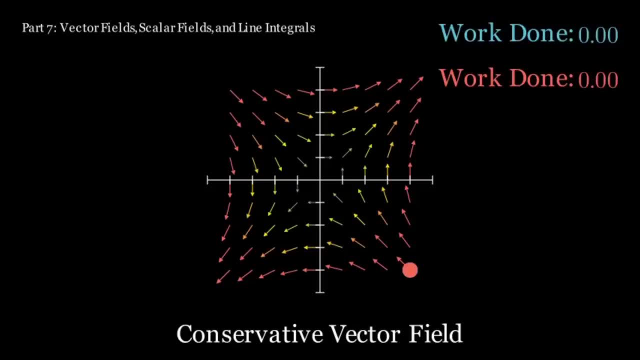 Vector fields can be conservative, meaning that any line integral on them is path-independent. This is very analogous to conservative forces, ie gravity, where the work done on particles is path-independent And in fact, gravity has a vector field, although this field varies depending on the objects that are present. 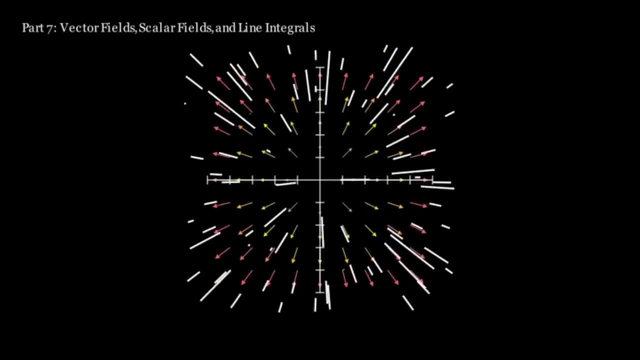 Vector fields have two main properties: divergence and curl. Divergence and curl are two main properties. Divergence and curl are two main properties. Divergence is the amount of outflow from a certain part of a vector field. In the center the divergence is high, since everything is moving outwards. 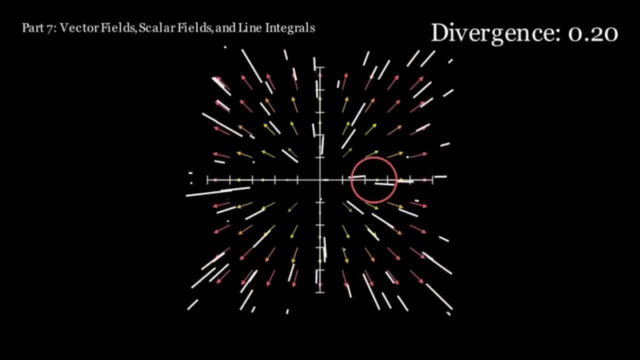 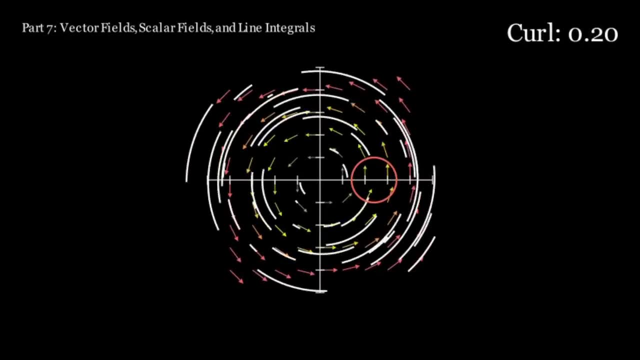 While further away the divergence is lower, since some points are moving in and some are moving out. Curl is the amount of rotation around a certain point in a vector field. Here, on the outside, the curl is low, since there is not much spin.